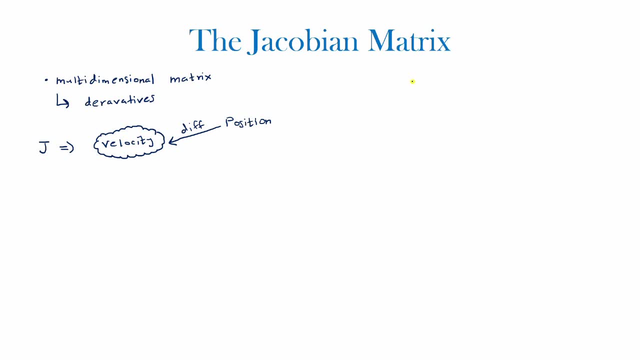 Let me give you an example. This can be generalized for almost any robot or any system involved in the Jacobian. You can have a general set of equations that describe the position of the joints in any system, such as: y1 equals f1,. some function with variables x1,, x2, and. 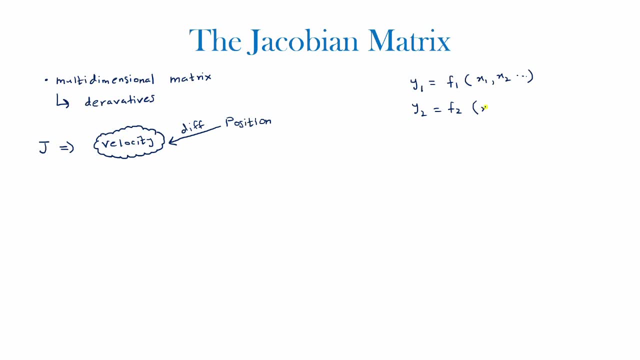 so on, Y2 would be f2. And you can have multiple equations, depending on the size of the system, which represent the position of the joints or the links in this robot When you take the differentiation or the derivative, and here you will be doing part of the question. 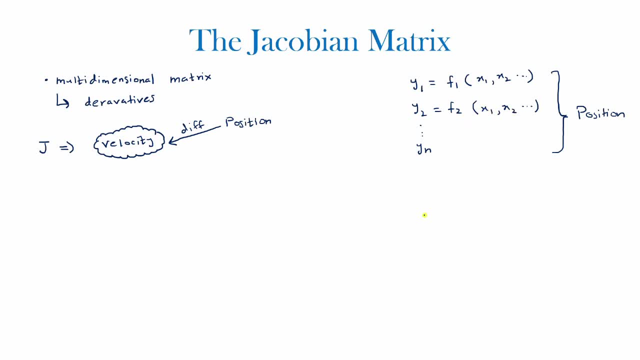 be doing partial differentiation because you have multiple variables in the function. you would get something that looks like daba y equals daba f over daba x times daba x, And this would actually be a matrix containing y1 dot, y2 dot and so on, Followed by the matrix holding the. 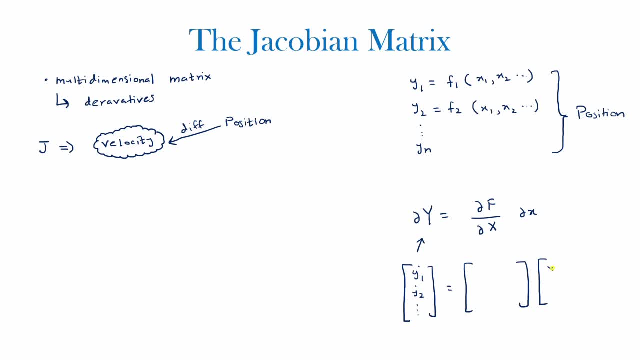 derivatives of the function times, the matrix holding x1 dot, x2 dot and so on. So this derivative of the function that correspond to this matrix and that matrix would be the Jacobian. Now I'm not going to go into detail on this because 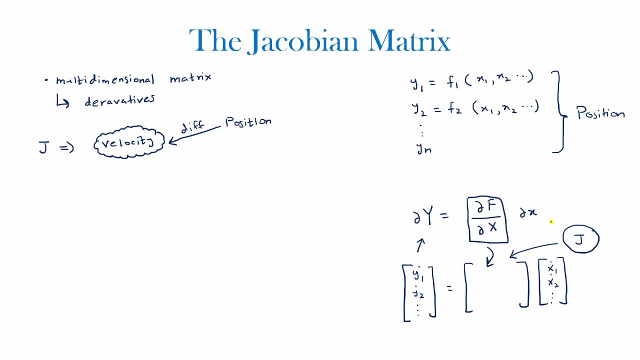 we will have a look at it again when we are doing partial differentiation in my next video. So let's keep this aside for now and let's have a look at the definition of the Jacobian. So the Jacobian can be used to relate the joint velocities to the Cartesian velocities. 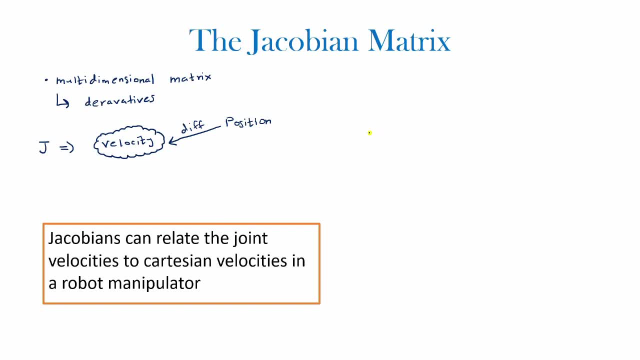 in a robot manipulator. So let me show you this in an equation format so it would be easy for you to understand. A joint or a link- usually a joint for a robot- can have a velocity. The velocity can be expressed in terms of the position vector for the three coordinates. 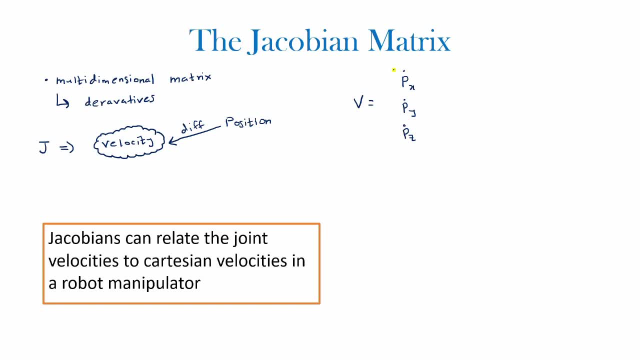 x, y, z, the derivative of those position vectors, And this would be the velocity in the Cartesian space. This would also be equal to the velocity in the joint space, which would comprise of two values, And this would be joint space, where v0 would be the linear velocity and omega would be 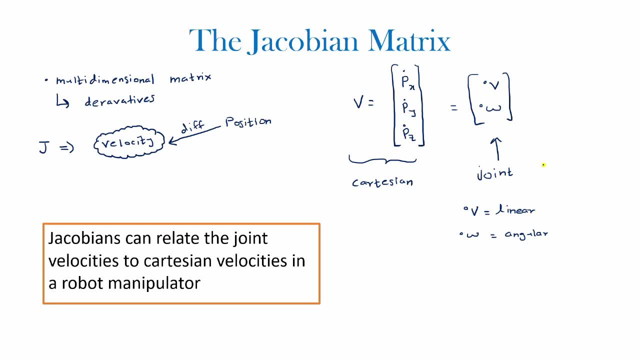 the angular velocity or the rotational velocity, And this would actually be equal to the Jacobian times, whatever variables are there in the system. I'm taking theta1 and theta2, for example, the derivatives of theta1 and theta2.. So the Jacobian can be used to relate the joint velocities to the Cartesian velocities. 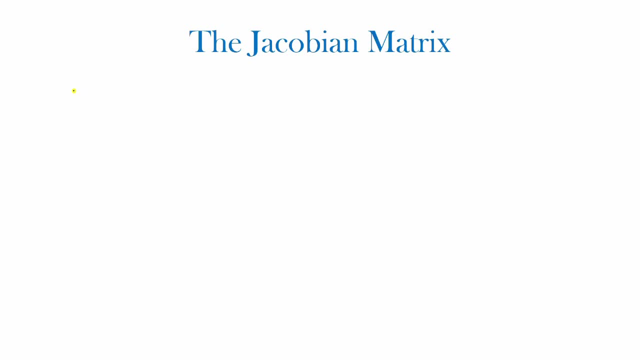 Right. so before we move on to the next topic, there is one more thing I would like to discuss, and that is the frame the Jacobian is in Now. just imagine a simple robot, sort of something like this, With a frame like this. 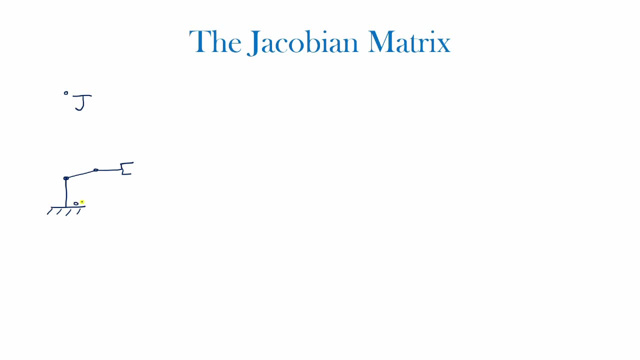 With a frame like this, With a frame like this, With the zeroth joint or the base frame being zero. This being the first frame, first joint, second joint and the third frame for the tool To perform most of the calculations involving torques, forces and singularities, you would. 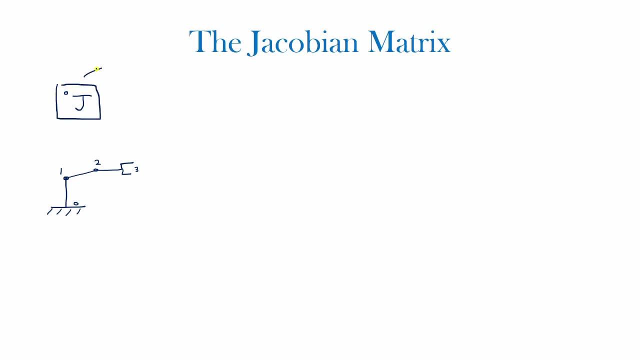 need the Jacobian in the base frame or J0. But when performing the calculations to find the Jacobian, you may end up with the Jacobian in the final frame, J3.. That being said, you can also express the Jacobian in any of the other frames as well. 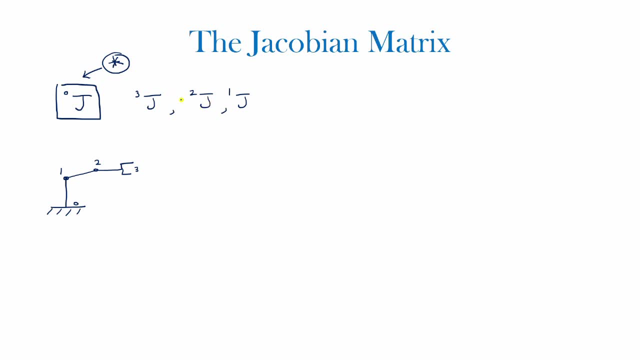 And from these other frames. we would need to use that value to find the Jacobian in the base frame. So how do you do that? Well, it's actually quite simple. The Jacobian in the base frame is equal to the rotation matrix from the base to any frame. 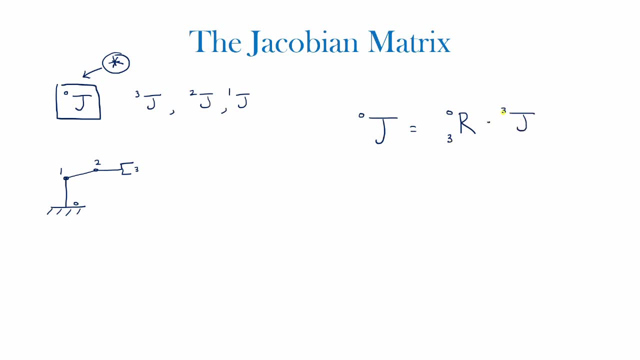 I'm using 3 here as an example- Times the Jacobian, The Jacobian in that particular frame. So you have to remember this equation. Practically, what you have to know is that if you have a Jacobian in the higher frame, 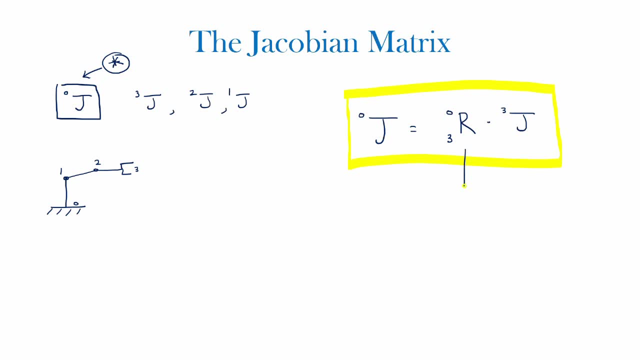 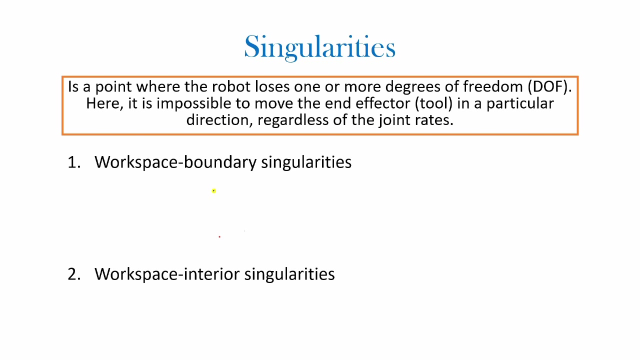 simply multiply it by its rotation matrix, which comes from the transformation matrix. So you have your position rotation. so you multiply it by the rotation matrix to get the Jacobian in the base frame. Alright, so now let's have a look at singularities. 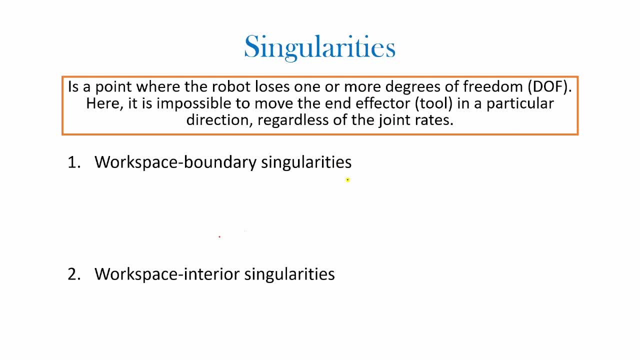 I'm not going to go into depth on this topic, but I will give you a brief introduction. By definition, a singularity is a point where the robot loses one or more degrees of freedom. At this point, it would be impossible to move the tool of the robot in a particular direction. 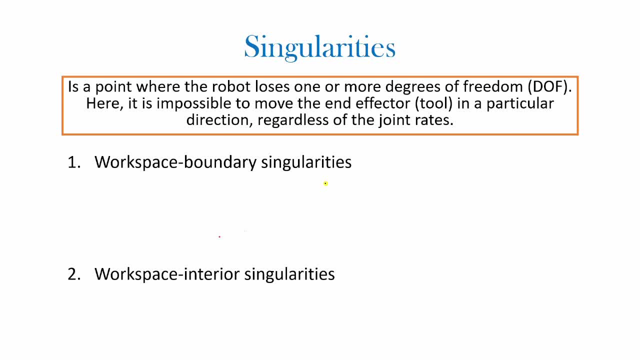 regardless of the joint rates. Now, there are two main types of singularities: workspace boundary and workspace interior. If you're not quite familiar with the term workspace, practically it means the area that the robot can operate in. So if this is the tool of the robot, it can operate within this entire frame. 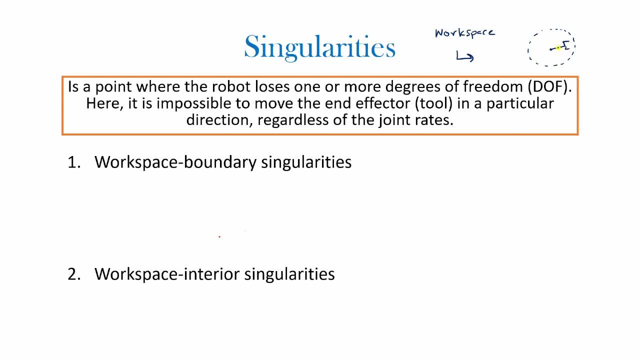 That's the area where the robot can operate. Okay, So it's going to be less than one degree in terms of space. It's going to be less than one degree in terms of space area and reach any object within this area. So that would be the workspace of. 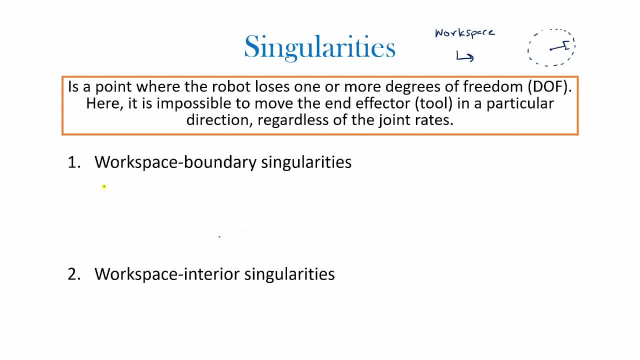 the robot. So for workspace boundary singularities, there are two cases, The first one being that the robot can either be fully stretched out or folded back on itself, And for both of these conditions the tool of the robot would be at the boundary of the workspace. In workspace interior singularities, the tool is no. 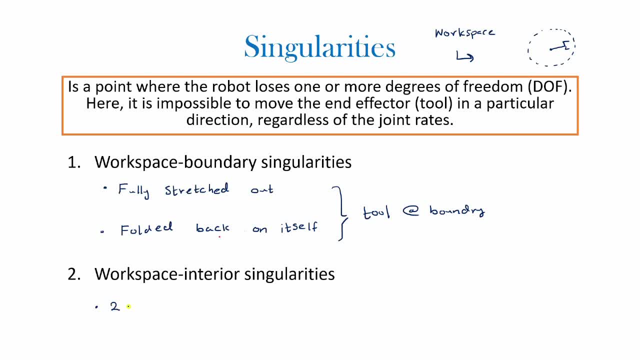 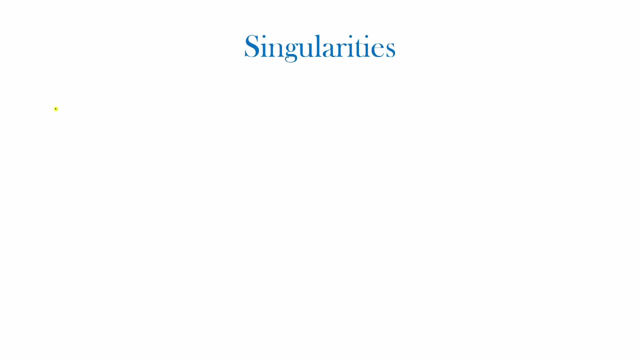 longer at the boundary, but two or more joint axes would line up with each other, So for this particular type of singularity to take place. So alright, so to help you visualize singularities, let's just take this example of a very simple robot with three joints, and this join can be: 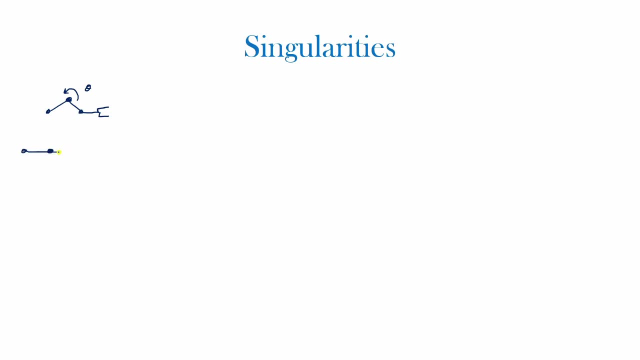 this robot or rotated that joint such that the robot was in a straight line. Here, theta would be equal to 180 degrees. At this point the robot has lost some degrees of freedom and therefore it is at a singularity. So the value theta equals 180 degrees would be the point at which the robot 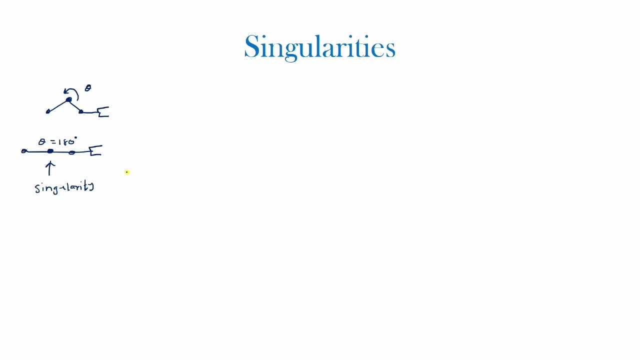 reaches its singularity, and we would. it would be of interest to calculate singularities because we would know at what points the robot loses its degrees of freedom. so we can program it to not reach those particular angles or to not allow the joints to rotate those particular angles to stop it from. 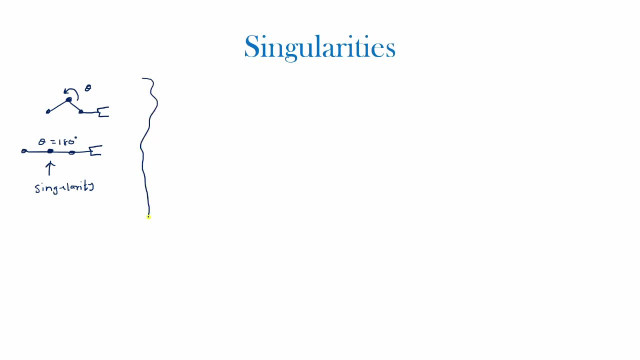 getting stuck, for example, Right. so to calculate or to find a singularity, you will look at the determinant of the Jacobian. So if the determinant of the Jacobian is equal to zero, then a singularity or singularities would exist for the robot. 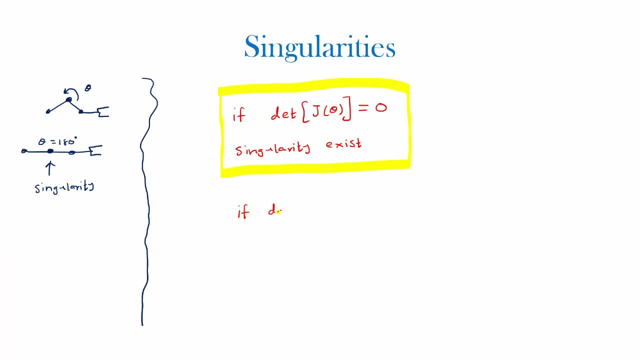 you. If, however, the determinant of the Jacobian is not equal to zero, there would be no singularities for that robot system. Right, so these are two things that you have to keep in mind Now when performing calculations, if the question asks you to find the singularity of a robot system. 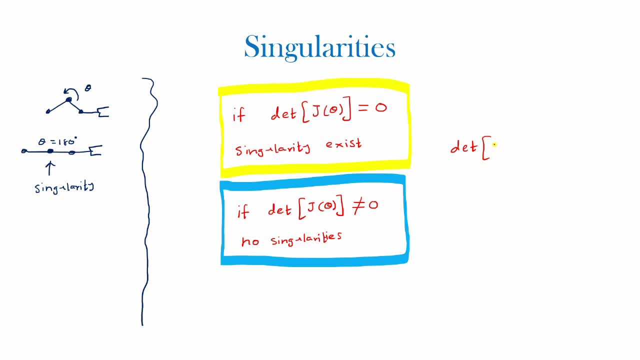 then you would find the determinant of the Jacobian and equate it to zero and you would get an equation with multiple different variables, such as theta 1, theta 2 and so on, And by equating this whole equation you would get a result. 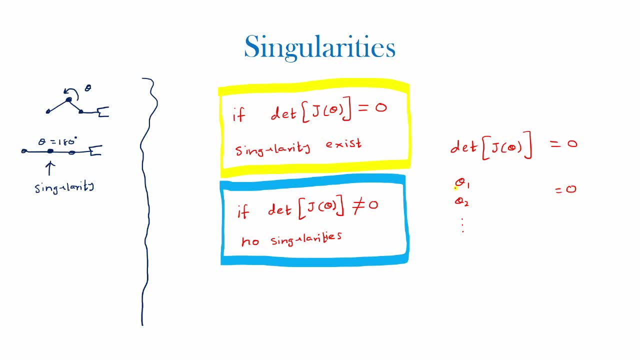 So if you were to equate this whole equation to zero, you would be able to calculate some values for theta 1, theta 2 or whatever the variables are there And those values. so just for example, as a theta 1 is 30 degrees, theta 2 is 60. 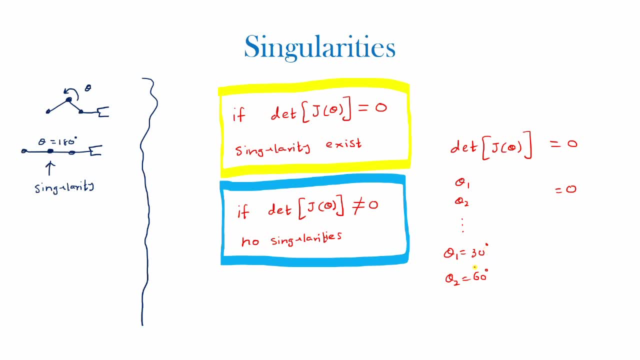 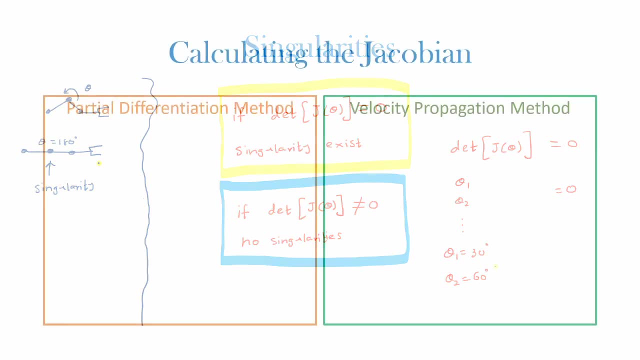 degrees. these values would be the singularities, so you would not want the robot or the joints to reach these particular angles. Alright, so now let's have a look at the two methods that we will use to find the singularities, To find the Jacobian. I'm not going to do any examples or explain this method in. 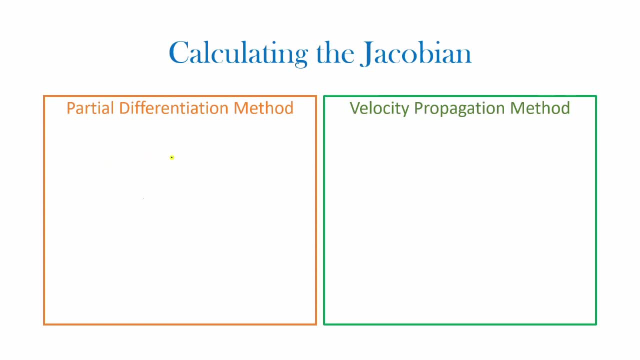 detail, rather just an introduction to each method, and I will go through each method separately in the following videos. So before we do that, just keep in mind that the Jacobian involves finding the velocity of the joints and the links of the robot Right. so the first method is the partial differentiation method. So 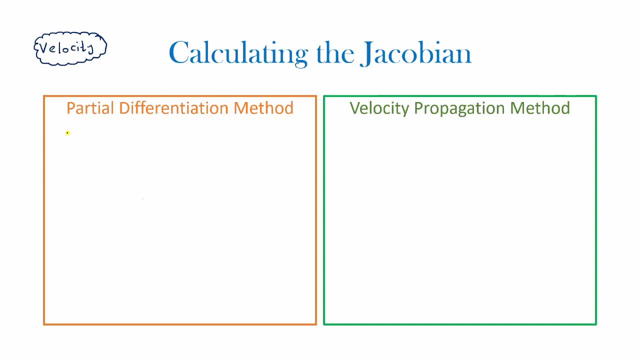 let's say we want to find the velocity of the joints and the links of the robot Right. so the first method is the partial differentiation method. So let's start from the very beginning. You have a robot, you assign your frames, you analyze, 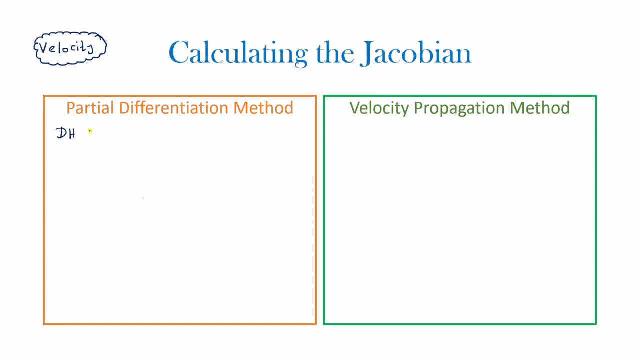 the system and you're able to form a DH table And from this DH table you would be able to get your transformation matrices. So you would have something at T01, T12 and so on And you see these transformation matrices. you can calculate the transformation matrix from. 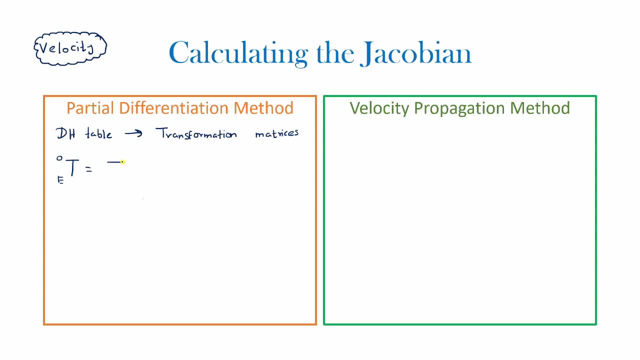 0 to the tool or the end effector, by multiplying all the previous transformation matrices together, 1 to 2, and so on, until you have N to E, And this final transformation matrix would be in the form of a 4x4 matrix. 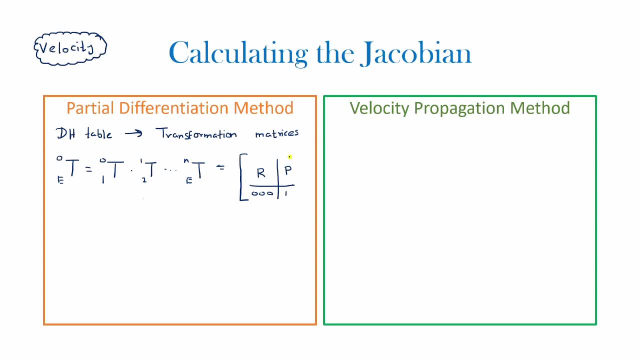 With a position vector and rotation matrix. So this position vector here would comprise of three values. You would have a position in x, y and z. So this would be the position of your end effector relative to your base frame. And if you were to differentiate each of these three and 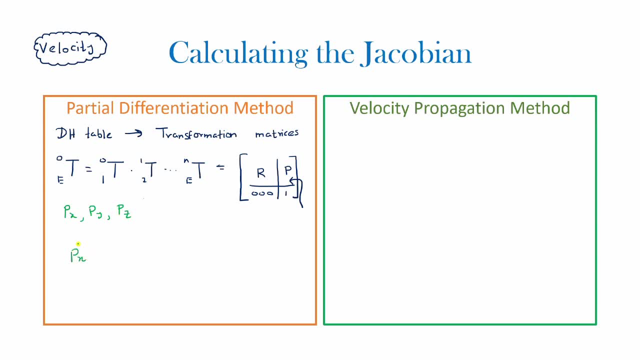 combine it to a matrix, you would have px, dot, py dot and pz dot and the equations that you get can be factorized into the form of the Jacobian relative to the base frame and whatever the variables were there in the equations, for example theta 1, theta 2 and theta 3. so in this case you can directly calculate the. 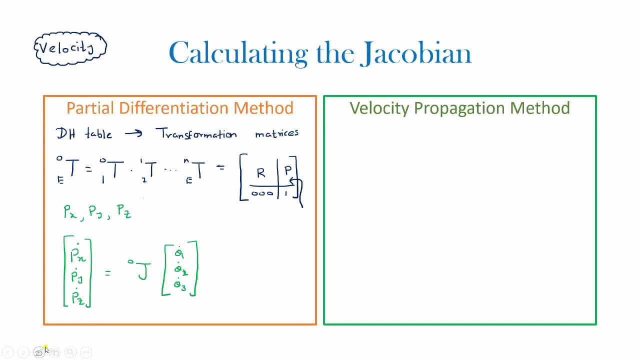 Jacobian in the base frame. now let's have a look at the velocity propagation method. so in the velocity propagation method you would first need to find the linear velocity denoted by V. then you would need to calculate the angular velocity denoted by Omega, keeping in mind that some 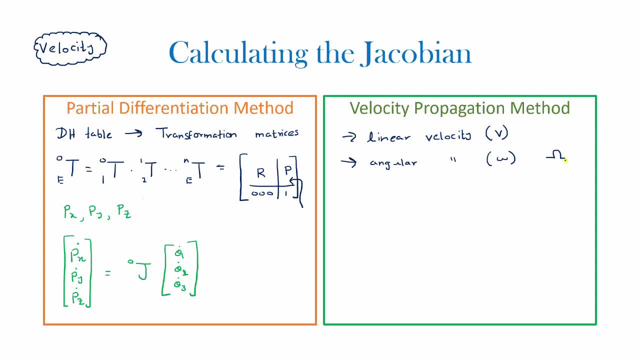 people or some textbooks would use this to denote the angular velocity, this symbol and there are already equations that you can use straight away to calculate the linear and angular velocity. you do not really have to take any derivatives or do any sort of differentiation, as the name suggests. 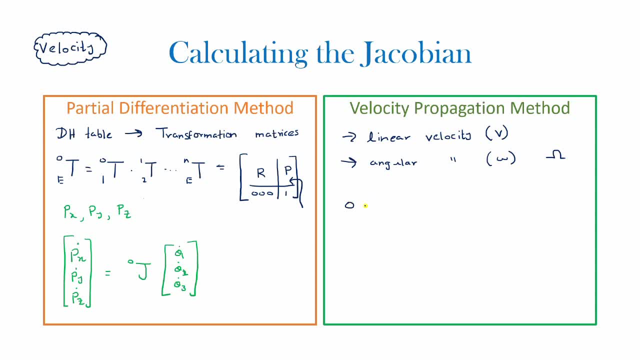 velocity propagation method. you start from the first frame, or the 0th frame, and work your way up frame by frame until you reach the final frame or the tool frame. so here you would finally have the velocity in the tool frame, and that velocity would be equal to the. 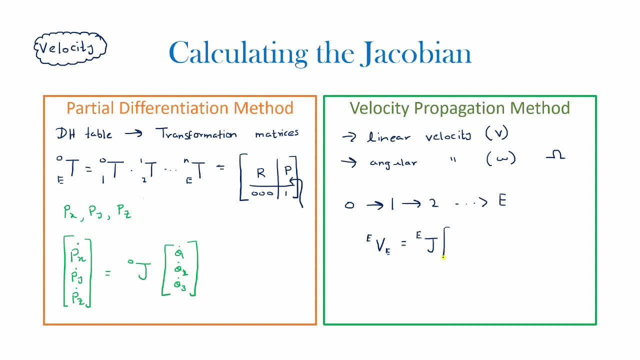 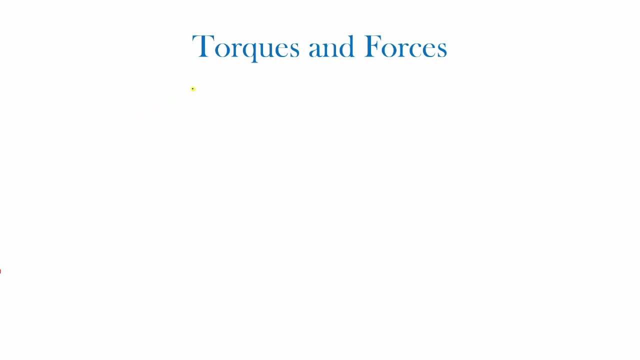 Jacobian in the tool frame times, whatever variables you had in your system. so from this we can calculate the Jacobian in the base frame using the rotation matrix from the base frame to the tool frame times the Jacobian in the tool frame. alright, guys. so the final thing we're going to look at in this video would be: 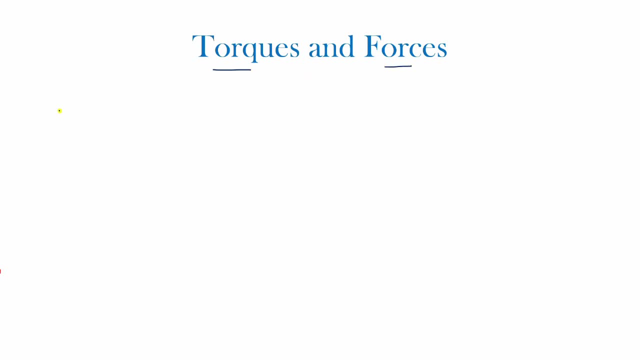 talks and forces. so we have two main types of joints that we looked at in this course. we had revolute joints and prismatic joints. so revelure joint would actually produce, or rotation, and so there would be a torc, while a prismatic joint would produce some sort of force. so, for example, we had 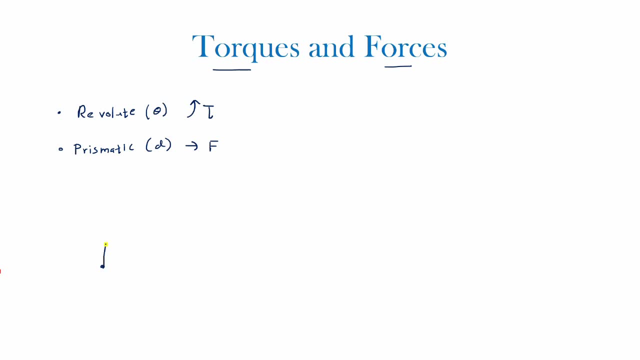 undefined system like this with two revolute joints and one prismatic joint. you would have two torques in this system: tau 1, tau 2. I better use a different color- tau 1, tau 2- and a force from the prismatic joint f3. so you can relate the. 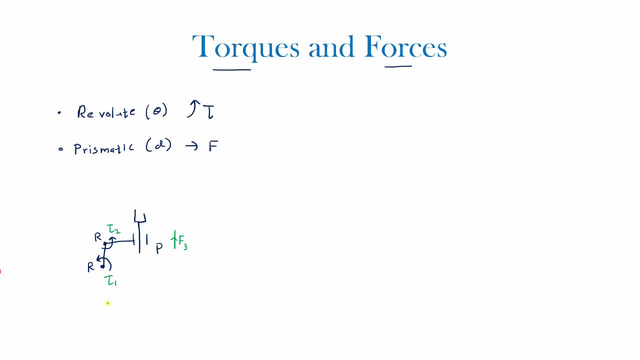 forces and the torques to each other by using a Jacobian, and that is done using this general equation is equal to the Jacobian from the base frame, the transpose of that Jacobian times F. So what you would actually get from this is related to this particular robot system. You would have tau 1,, tau 2, and F3 equal.